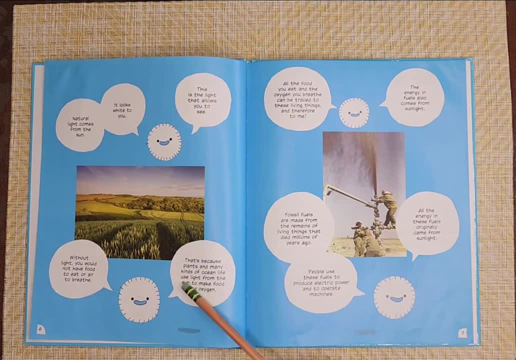 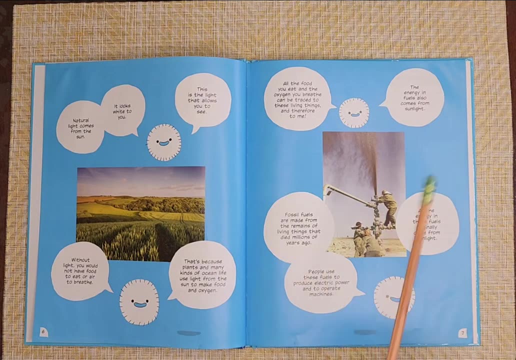 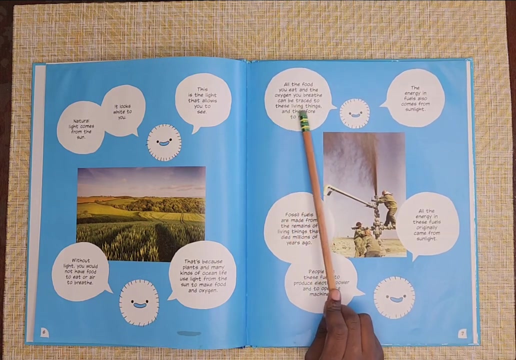 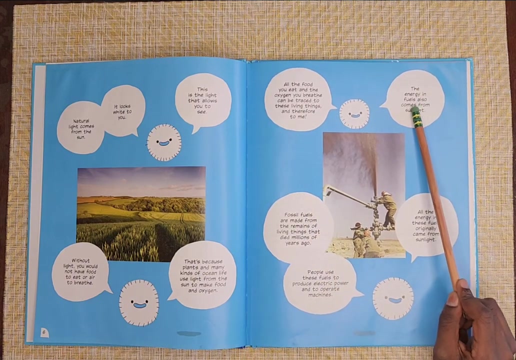 That's because plants and many kinds of ocean life use light from the sun to make food and oxygen. All the food you eat and the oxygen you breathe can be traced to these living things and therefore to me. The energy in fuels also comes from sunlight. 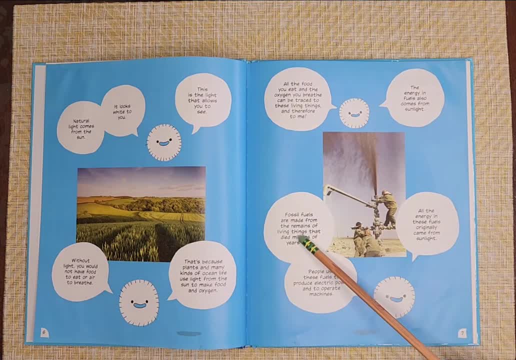 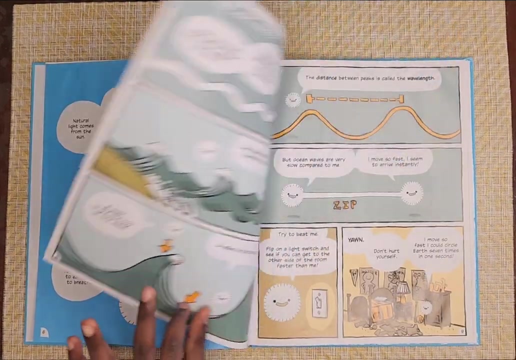 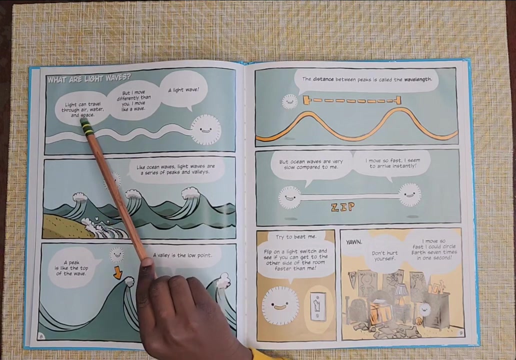 Fossil fuels are made from the remains of living things that died millions of years ago. People use these fuels to produce electric power and to operate machines. All the energy in these fuels are originally came from sunlight. What are light waves? Light can travel through air, water and space. 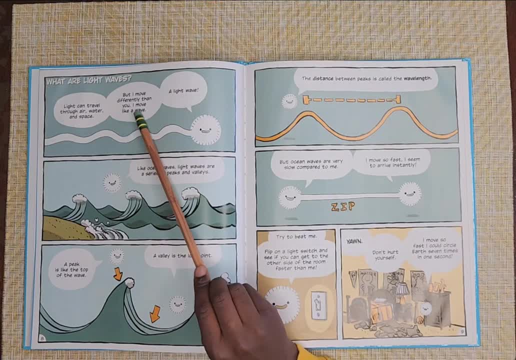 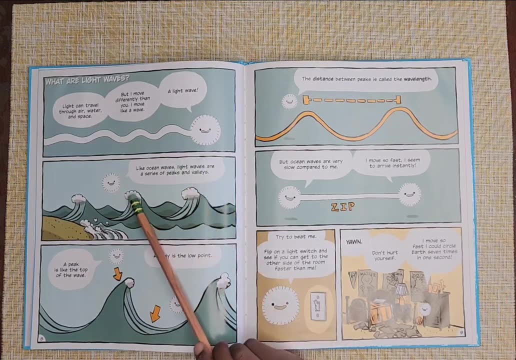 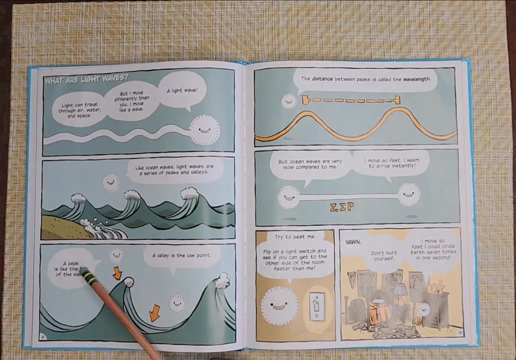 I move differently than you. I move like a wave, a light wave, like an ocean wave. Light waves are a series of peaks and valleys. A peak is like the top of the wave. A valley is the low point. Do you see the peak? 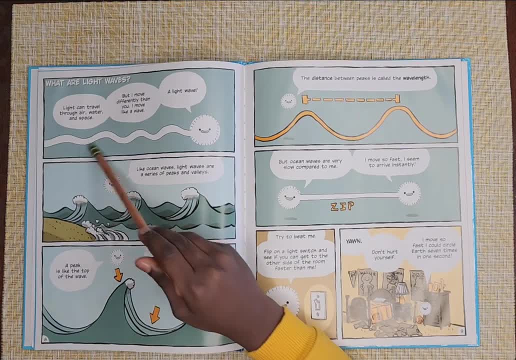 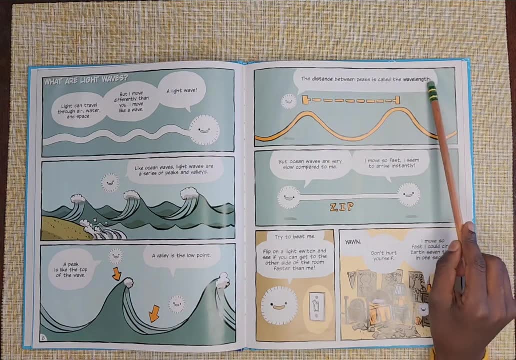 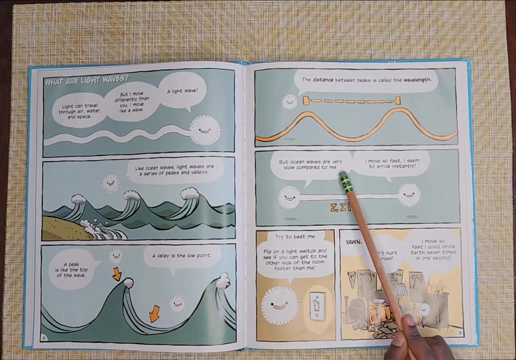 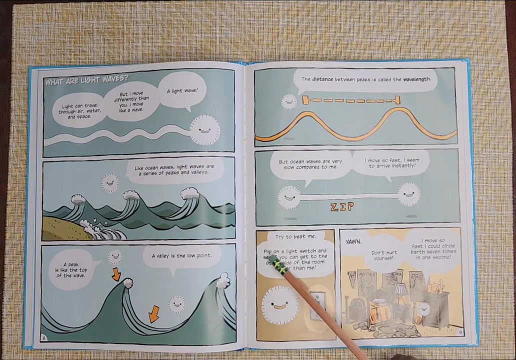 Do you see the low point? Do you see the wave? The distance between peaks is called the wavelength. See, But ocean waves are very slow compared to me. I move so fast I seem to arrive instantly. Try to beat me. Flip on the light switch and see if you can get to the other side of the room faster than me. 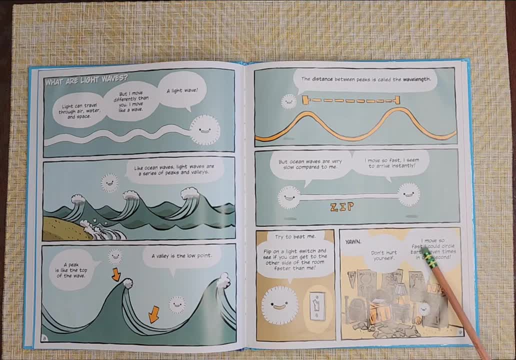 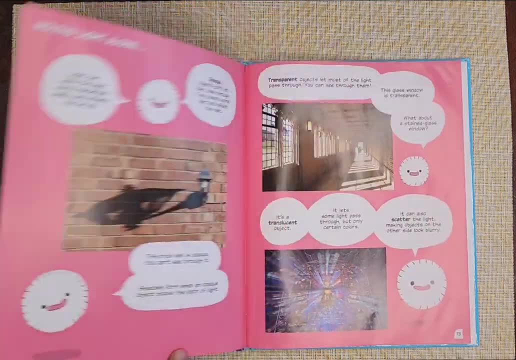 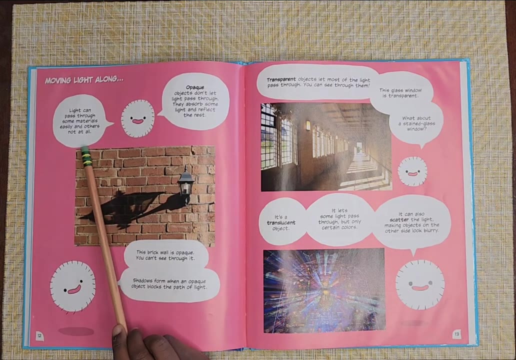 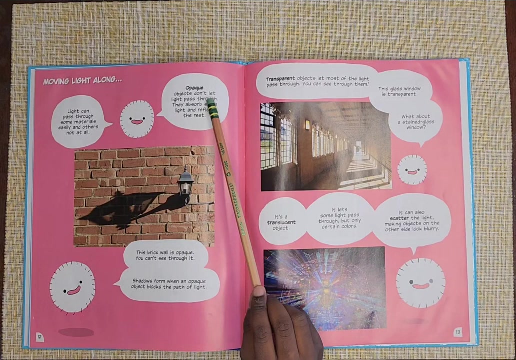 Don't hurt yourself, I can move so fast. I could circle Earth seven times in one second. Light can pass through some materials easily And not. Uh, there's not at all Opaque, Opaque. I just don't let light pass through. 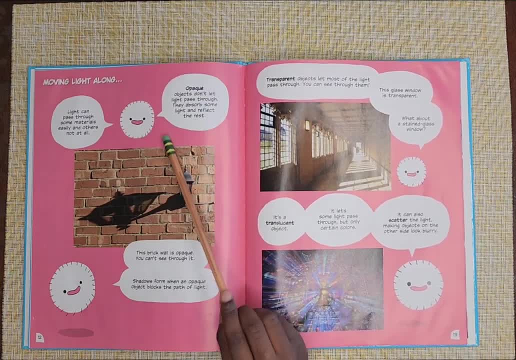 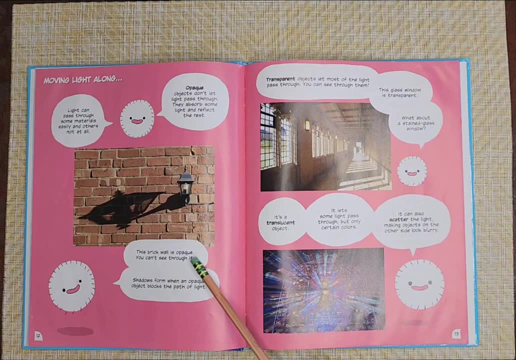 They absorb some light and reflect the rest. See, The brick wall is op, okay, opeque, huh, ہمممممممممممممممممممممممممممممممممممممممممممممممممの hä ああああああああああ. 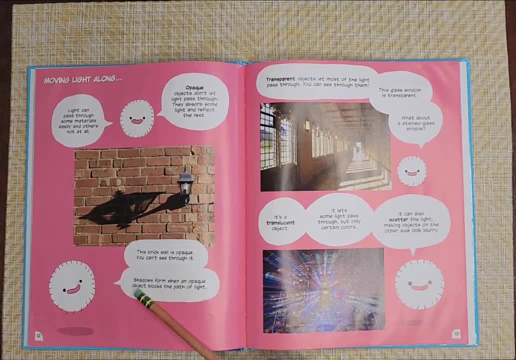 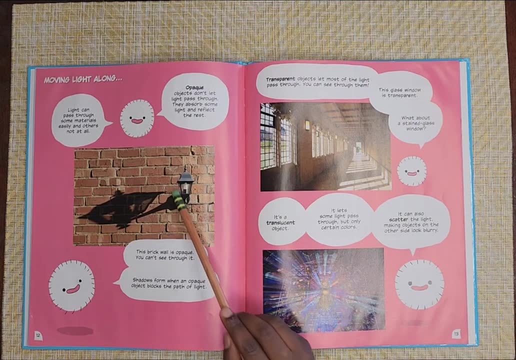 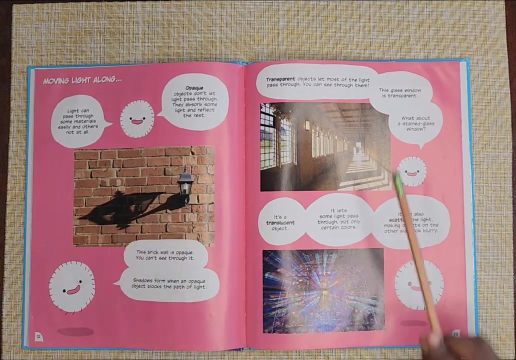 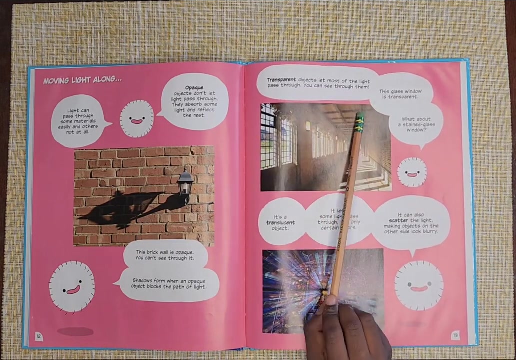 Opaque, You can't see through it. Shadows form when opaque objects block the path of light. See, The shadow is blocked. Only the glass is. clear, Transparent objects let most of the light pass through. You can see through them. This glass window is transparent, See, Some light is passing through easily. 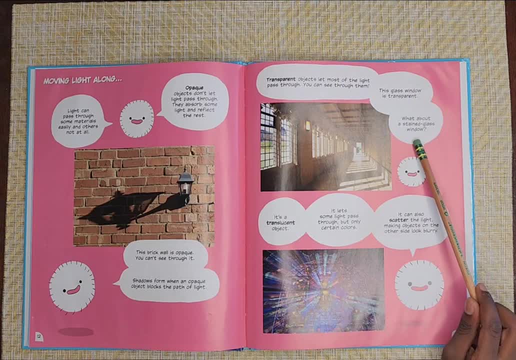 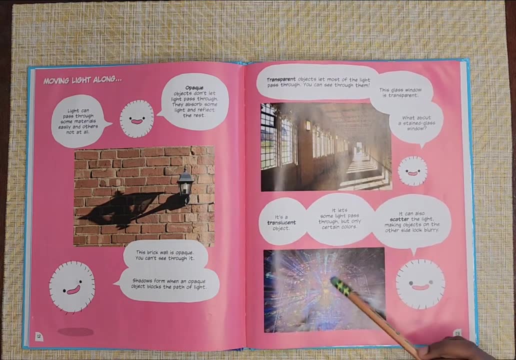 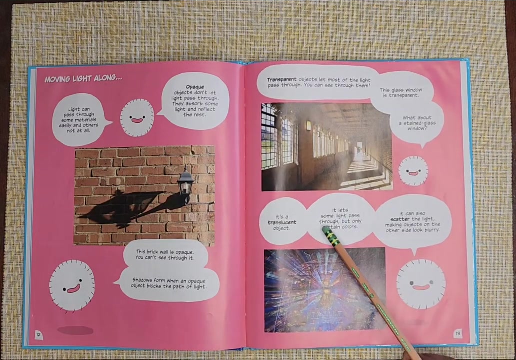 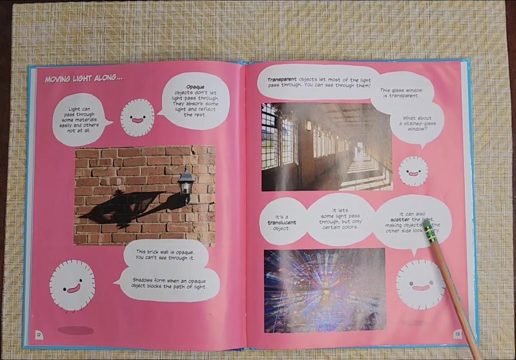 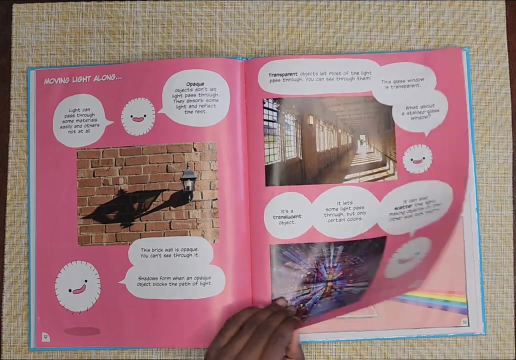 What about a stained glass window? It's a translucent object. See, It's a translucent object. It lets some light pass through, but only certain colors. See, It can also scatter the light, making objects on the other side look blurry. 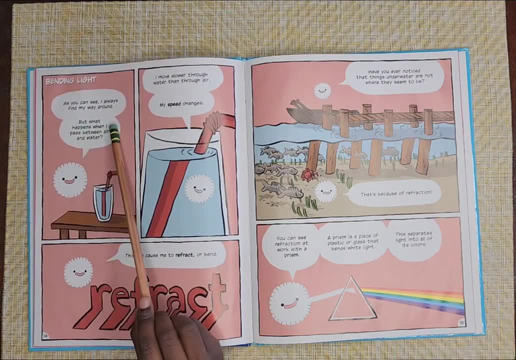 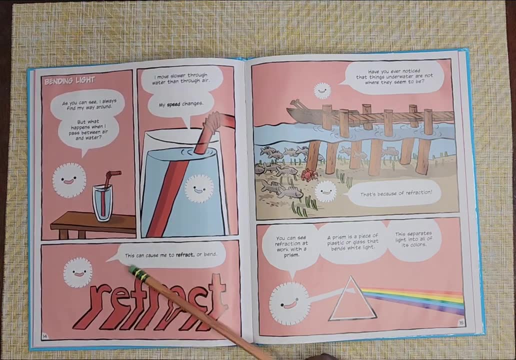 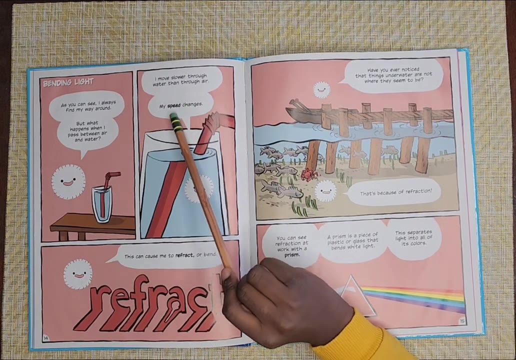 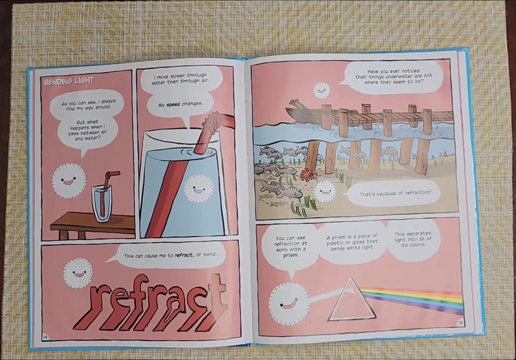 As you can see, I always find my way around. But what happens if I move? When I pass between air and water, I move slower through water than through air. My speed changes. This can cause me to refract or bend. Maybe next time we can do this experiment. 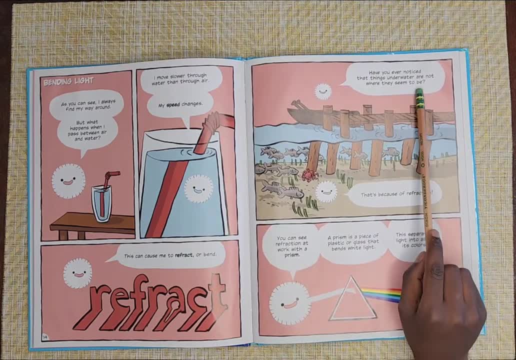 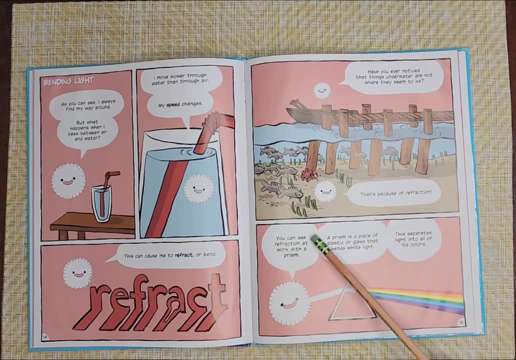 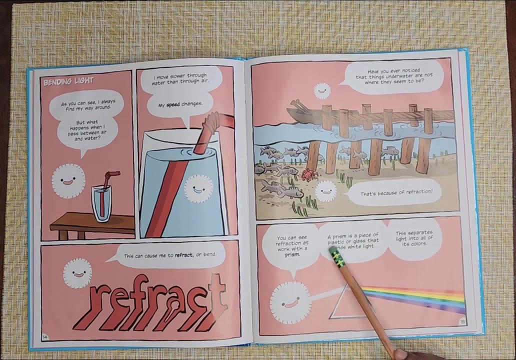 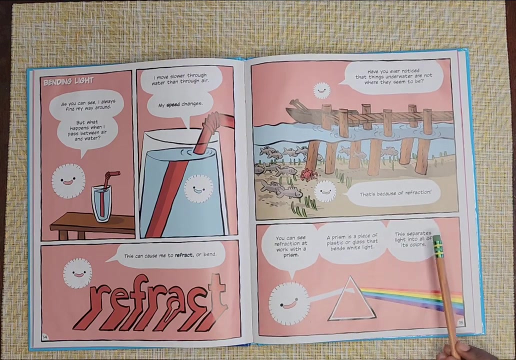 Have you ever noticed that things underwater are not where they seem to be? That's because of refraction. You can see refraction at work with a prism. A prism is a piece of plastic or glass that bends white light. See, This separates light into all of its colors. 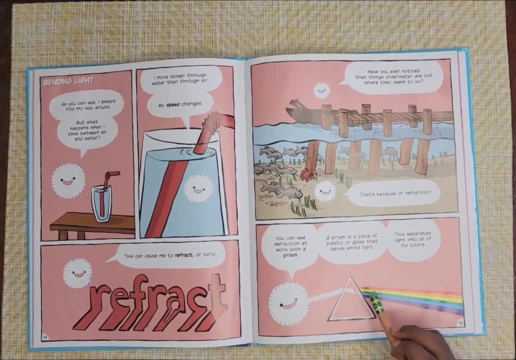 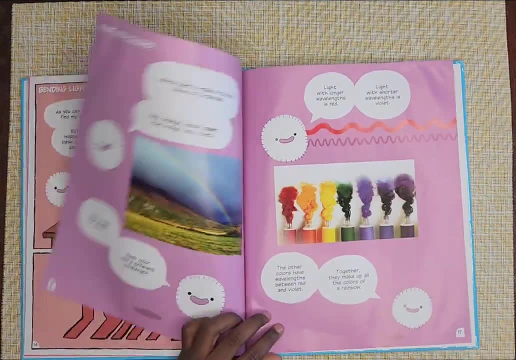 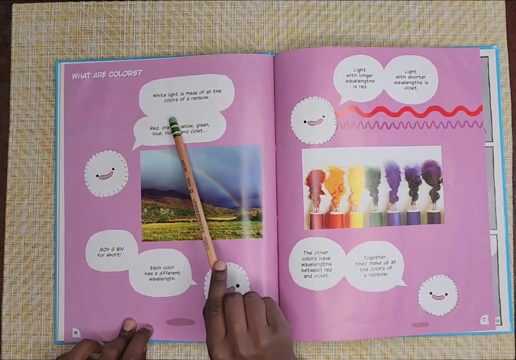 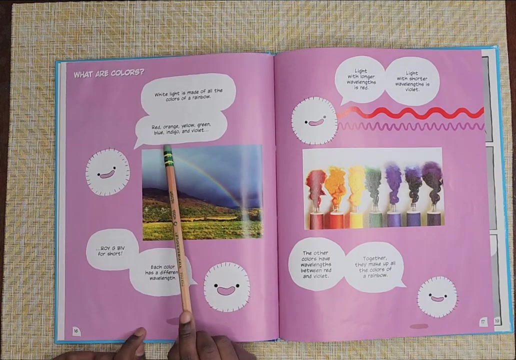 We can also do this experiment too. Do you see the rainbow? That looks cool. What are colors? White light is made of all the colors of a rainbow. Wow, Do you see the beautiful rainbow? Red, orange, yellow, green, blue, indigo and violet. 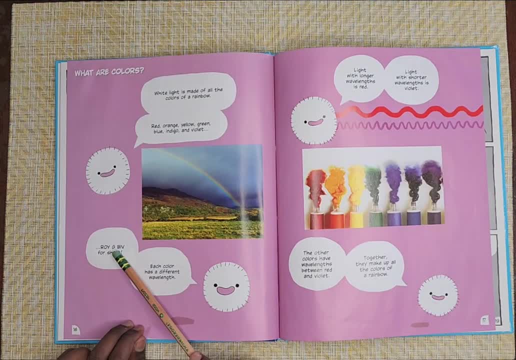 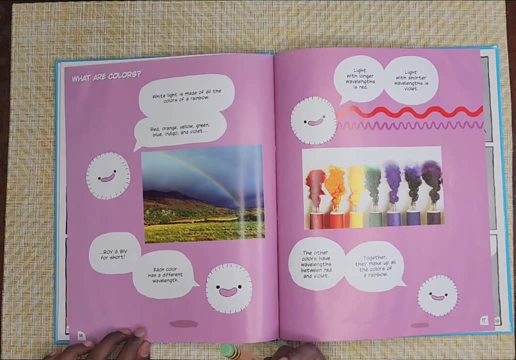 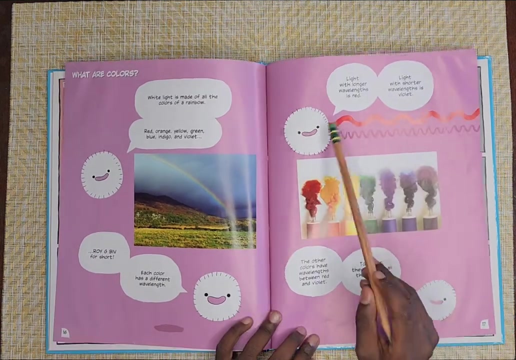 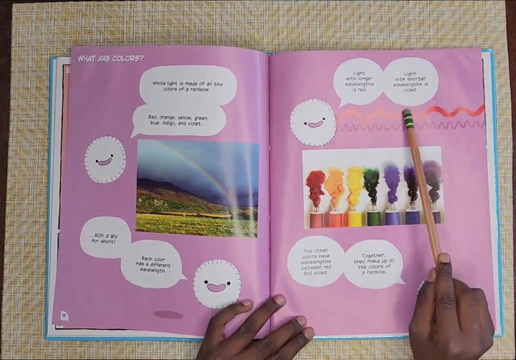 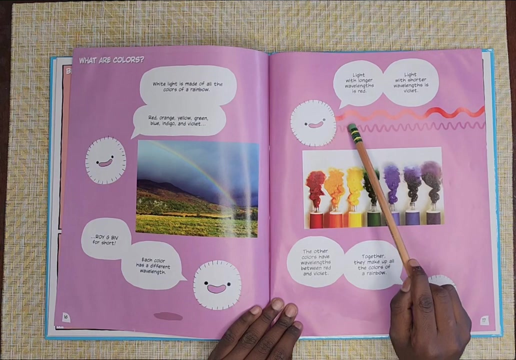 Or Roy Gibbett for short EVGR, for another way to say rainbow. Each color has a different wavelength. Light with longer wavelengths is red- See, It's so thick. Light with shorter wavelengths is violet: It's so thin. 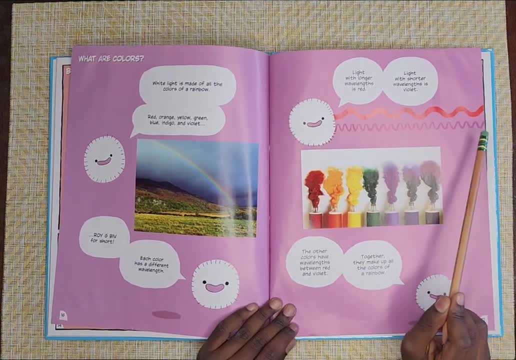 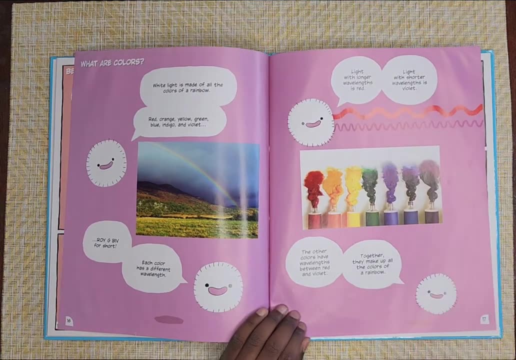 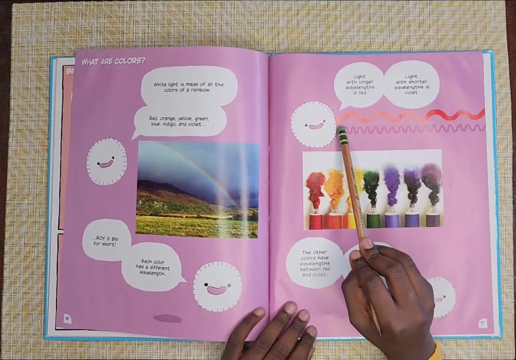 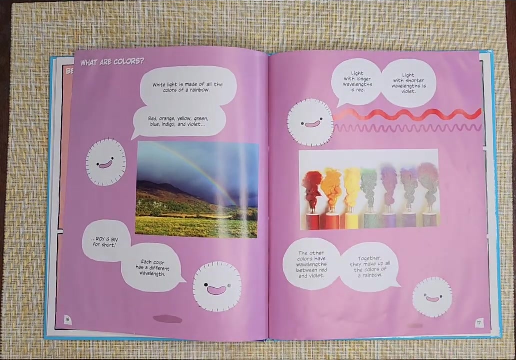 And it has a very much bends, But it's super-duper small And the wavelength is super-duper small. The distance to the peak is very small, But red has a distance to the peak very big. That's why it's big. 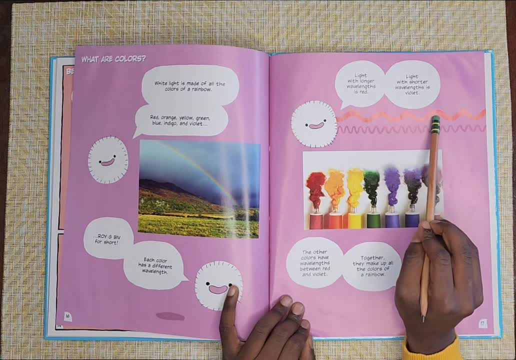 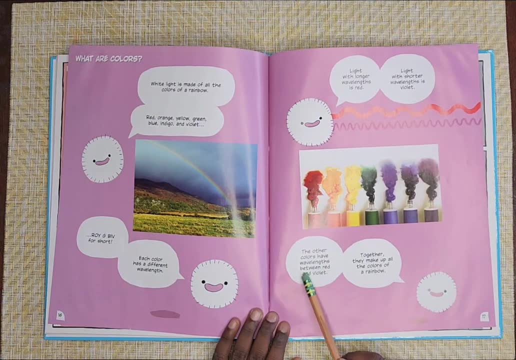 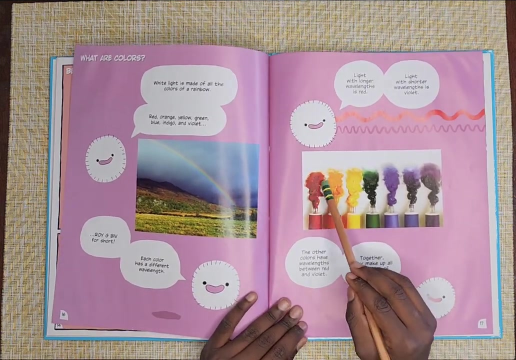 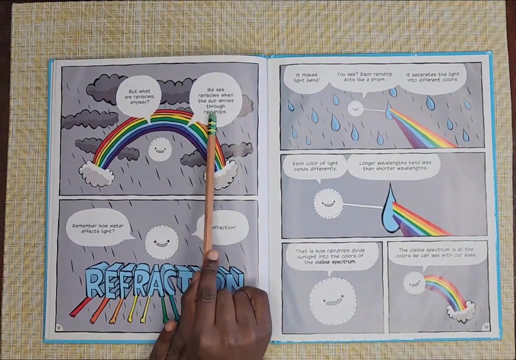 And also it has very big bends. The other colors have wavelengths between red and violet. Together they make up all the colors of a rainbow. See, These are all the colors, But what are rainbows anyway? We see rainbows when the sun shines through raindrops. 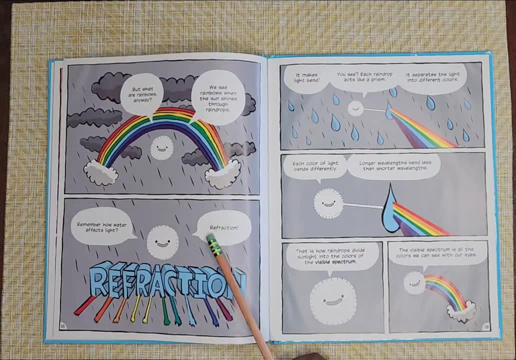 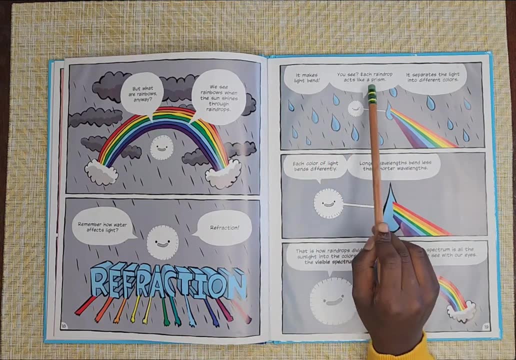 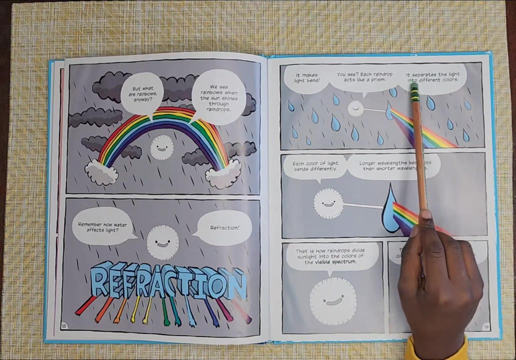 Remember how water affects light Refraction. It makes light bend. You see, Each raindrop acts like a prism. Wow, It separates the light into different colors of the rainbow. Each color of light bends differently. Longer wavelengths bend less than shorter wavelengths. 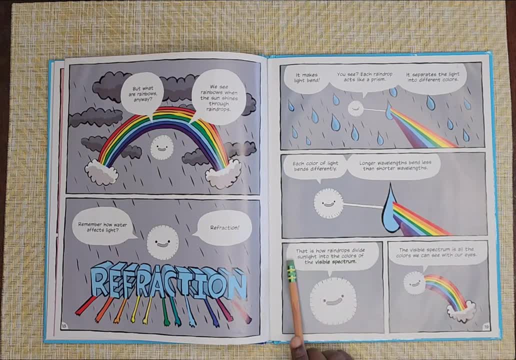 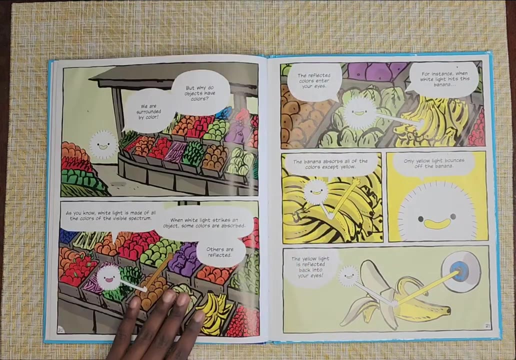 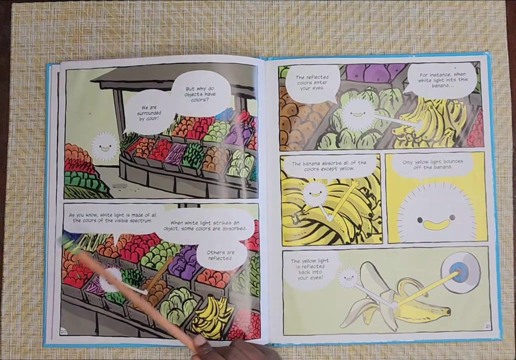 That is how raindrops bend. Now, raindrops divide sunlight into the colors of the visible spectrum. The visible spectrum is all the colors we can see with our eyes. We are surrounded by color. But why do objects have color? As you know, white light is made of all the colors. 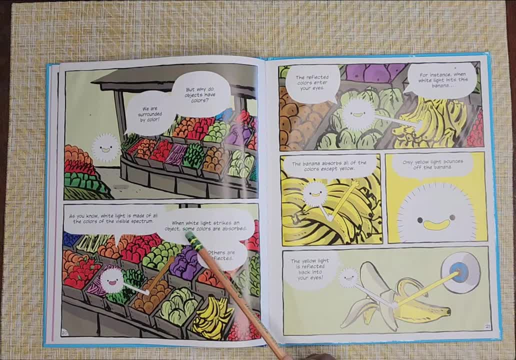 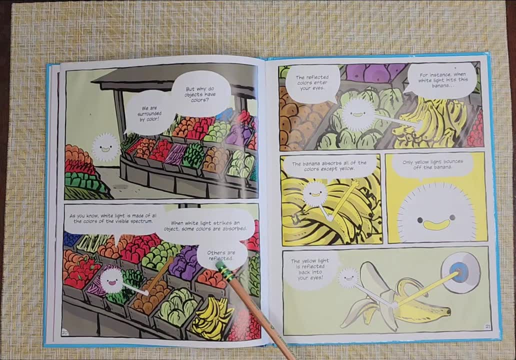 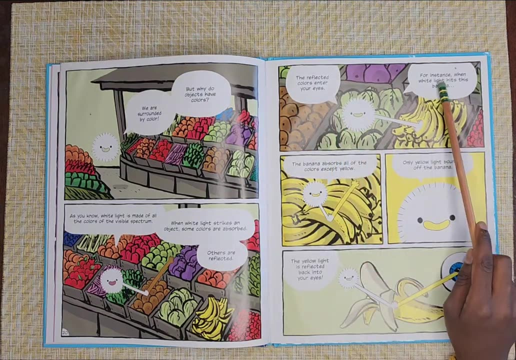 of the visible spectrum. When white light strikes an object, some colors are absorbed, Others are reflected. The colors reflected enter your eyes. For instance, when white light hits this banana, the banana absorbs all of the colors except yellow. See, It's getting out the yellow. 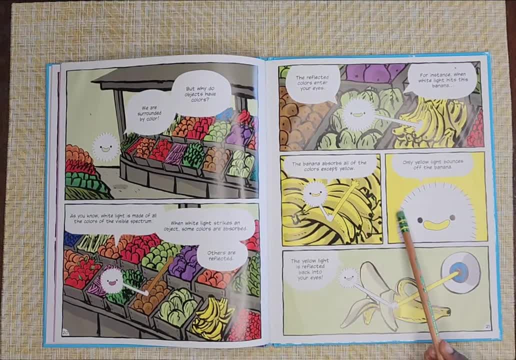 Like when you get a banana from the shop it's yellow, But then you can know it's actually not yellow. It's all the colors except yellow, Only yellow light bounces off the banana. The yellow light is reflected back into your eyes. 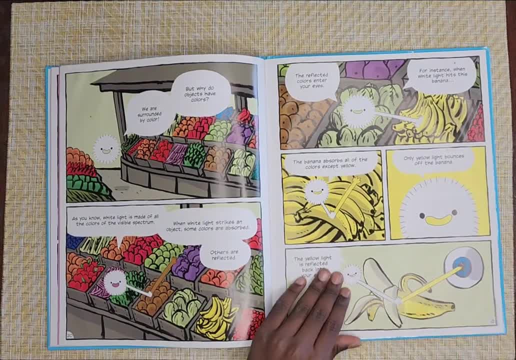 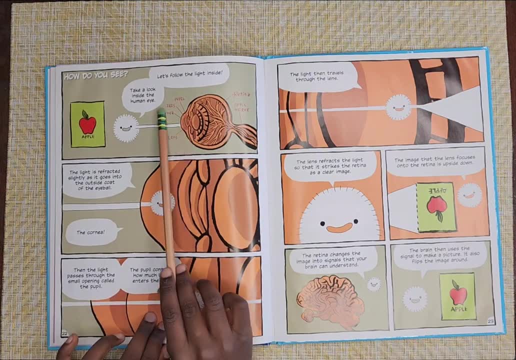 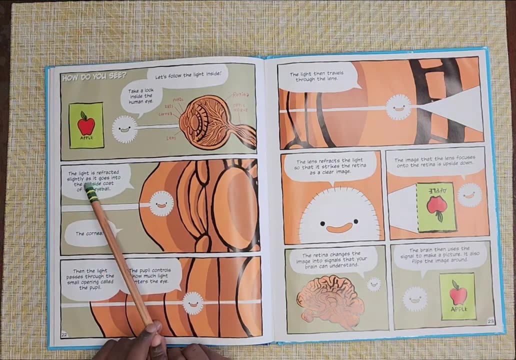 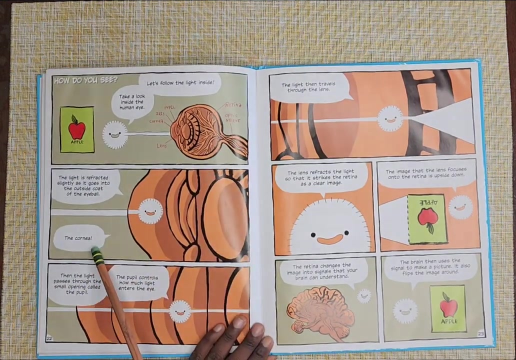 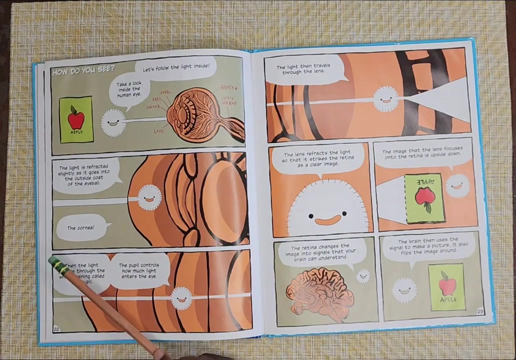 See, That's why it looks yellow. Let's follow the light inside. Take a look inside the human eye. The light is reflected slightly as it goes into the outside coat of the eyeball, The cornea, Cornea, Cornea. 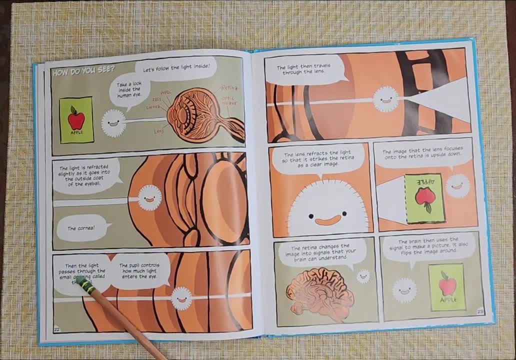 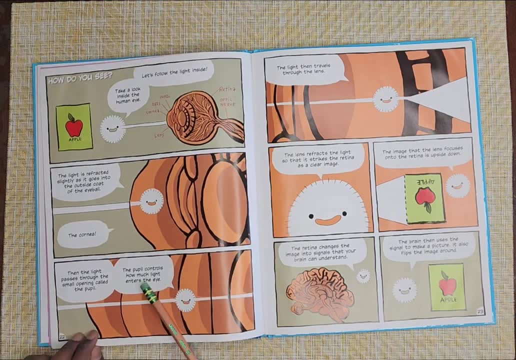 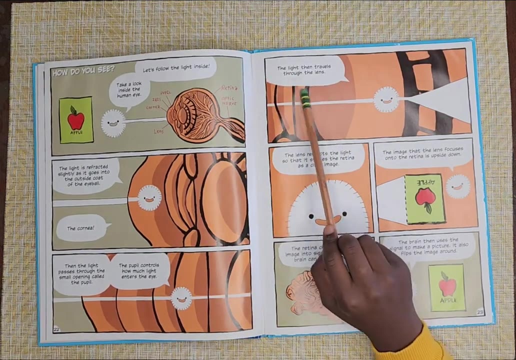 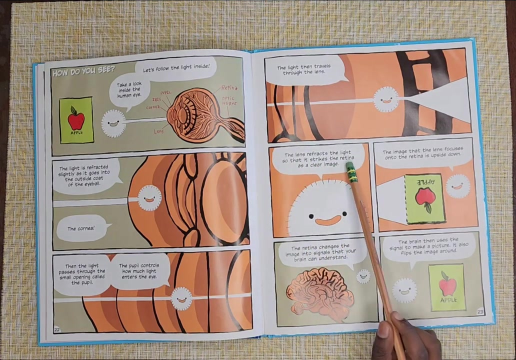 Cornea. Then the light passes through the small opening called the pupil. The pupil controls how much light enters the eye. Then the light travels through the lens. The lens refracts the light, so it strikes the retina. The retina has a clear image. 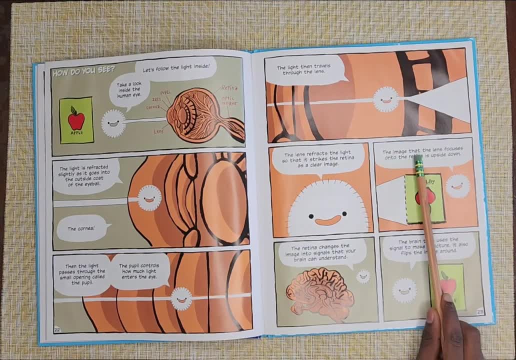 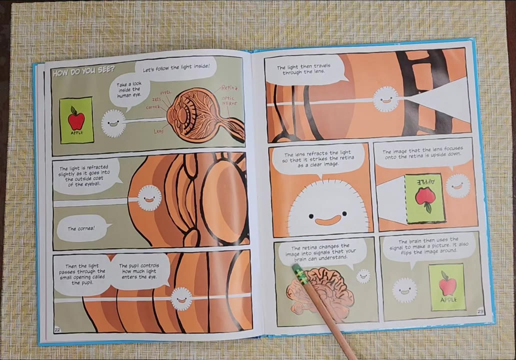 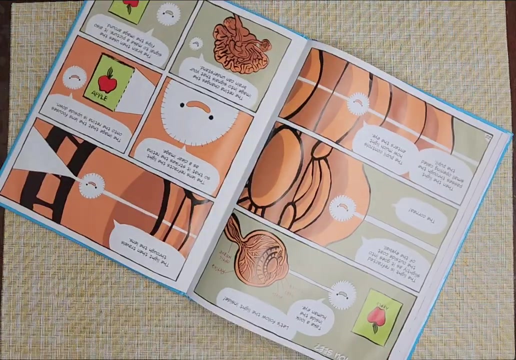 The image that the lens focuses onto the retina is upside down. The retina changes the image into signals that your brain can't understand. Wait, Can you see? the apple picture is upside down. Let's turn it upside down to see how it actually looks like. 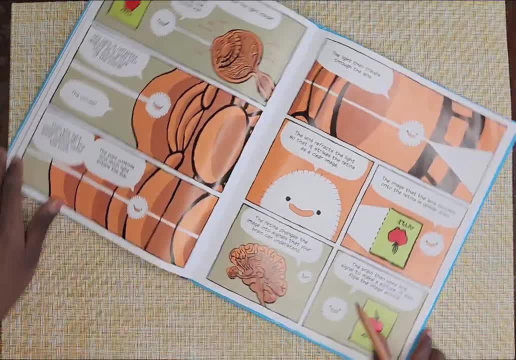 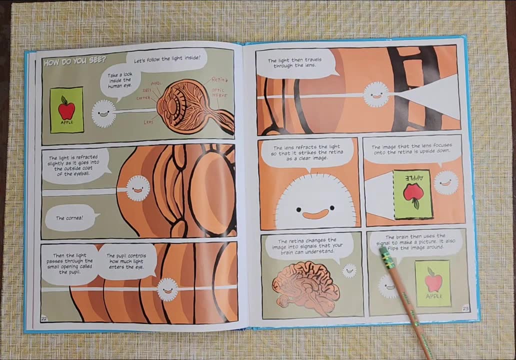 Ooh. The brain then uses the signal to make a picture. It also flips the image around. Oh, that's how it looks like. Wait, Your eyes see upside down. That's weird. Well, the brain makes it the right way. 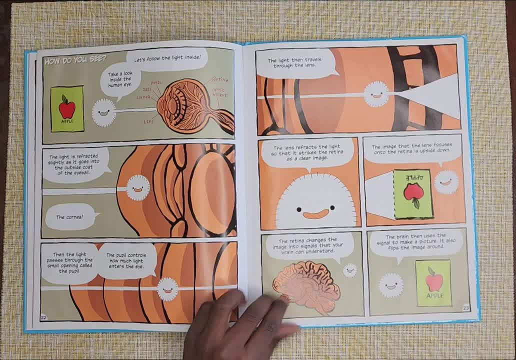 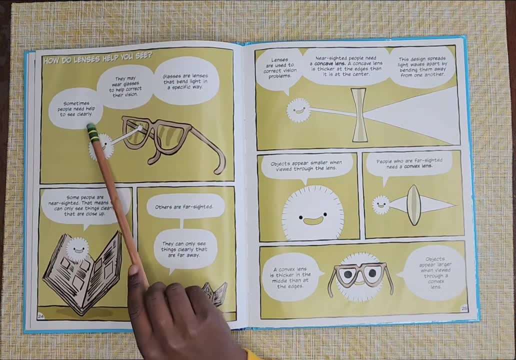 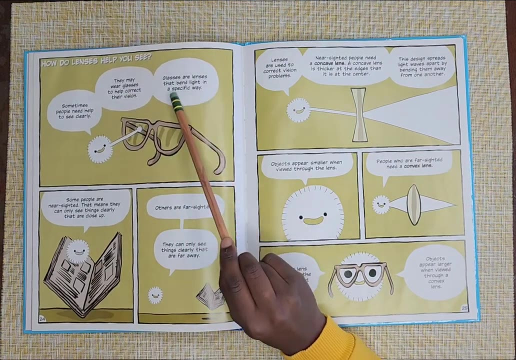 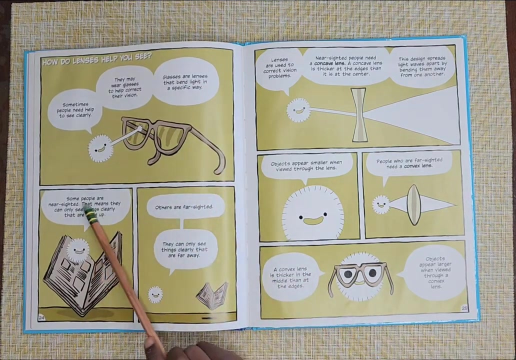 That's the right way, so that's good. Sometimes people need to see clearly. They may wear glasses to help correct their vision. Glasses are lenses that bend light in a specific way. Some people are nearsighted. That means that they can only see things clearly that are up close. 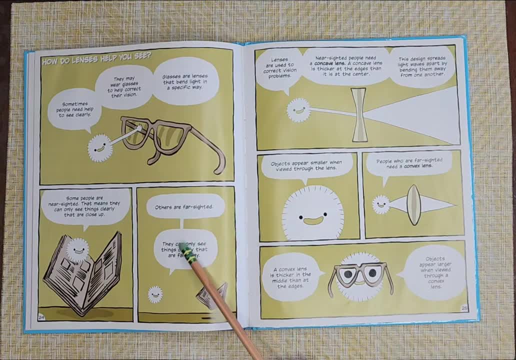 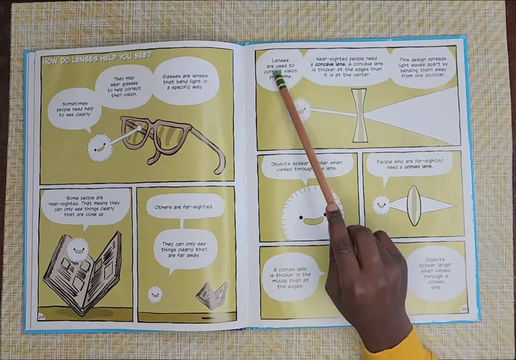 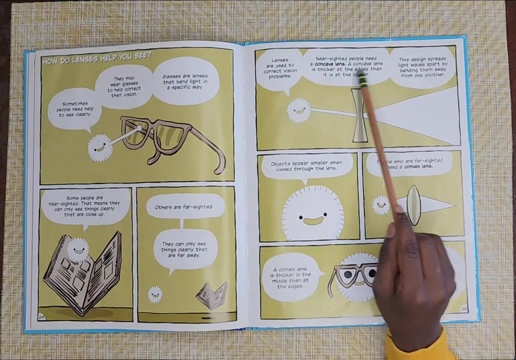 Some others are farsighted. They can only see things clearly that are far away. Lenses are used to correct vision problems. Nearsighted people need a concave lens. A concave lens is thicker at the edges than it is at the center. 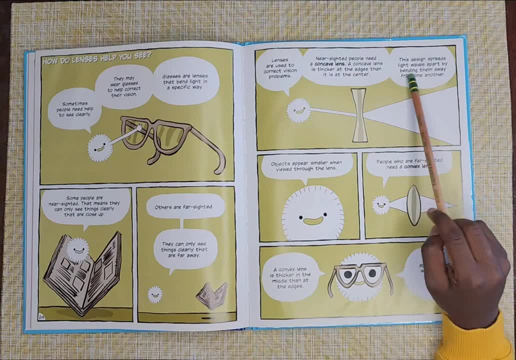 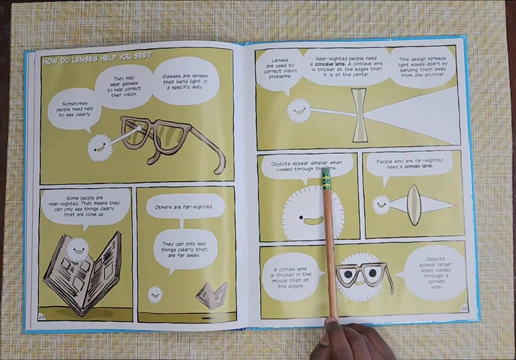 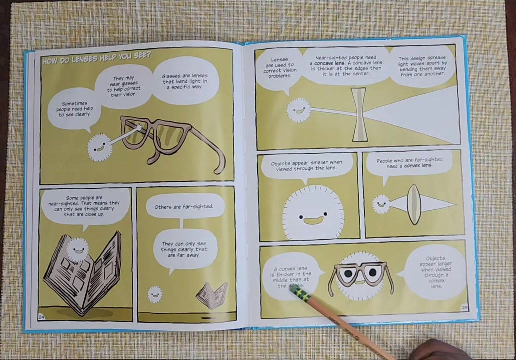 This device spreads light waves apart by bending them away from one another. Objects appear smaller when reviewed to the lens. People who are farsighted need a convex lens. A convex lens is thicker in the middle than at the edges. Objects appear larger when reviewed through a convex lens. 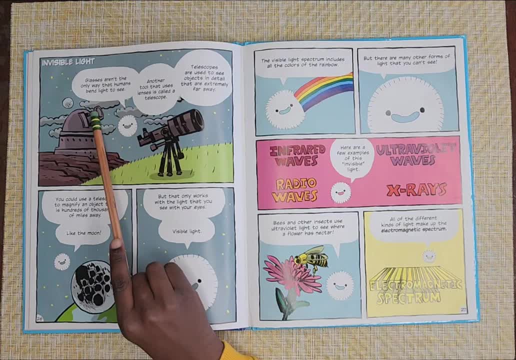 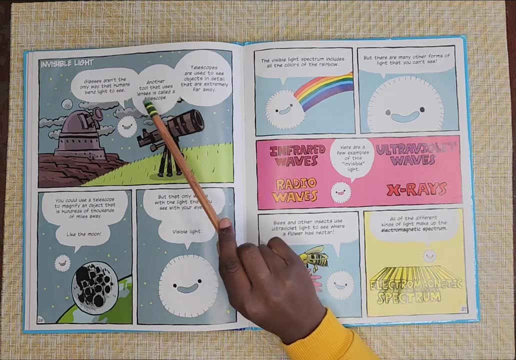 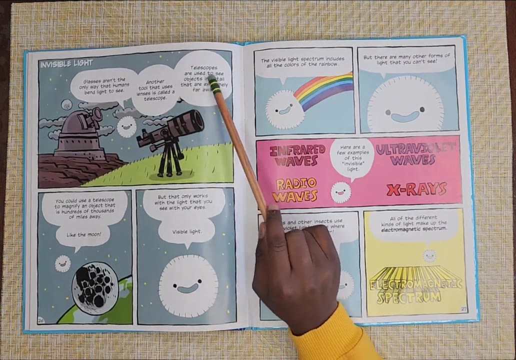 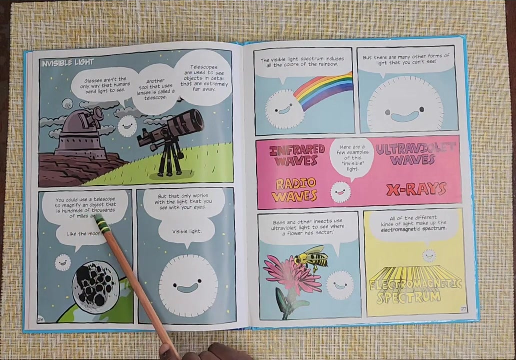 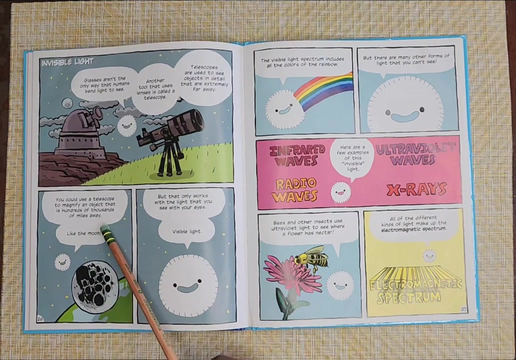 Glasses aren't the only way that humans bend light to see. Another tool is uses lenses. that is called a telescope. Telescopes are used to see objects in detail that are extremely far away. You could use a telescope to magnify an object that is hundreds of thousands of miles away, like the moon. 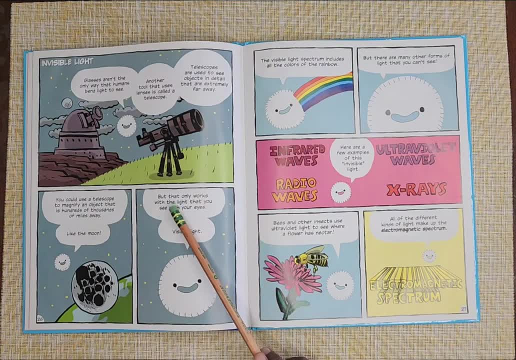 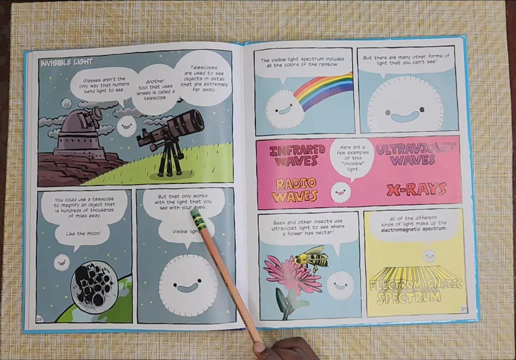 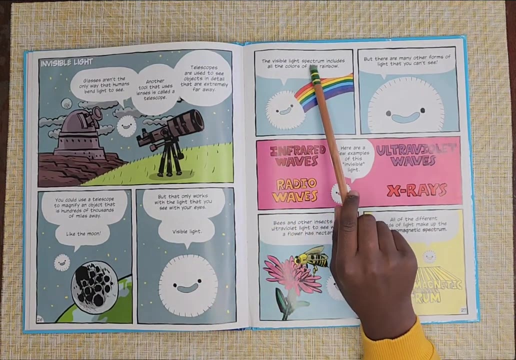 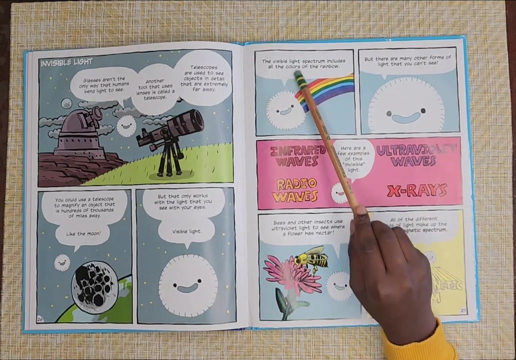 This is called invisible light. I forgot to say that. Sorry, But that only works with the light that you see with your eyes. Visible light, The visible light of spectrum, uses all the colors of the rainbow. Includes all the colors of the rainbow. 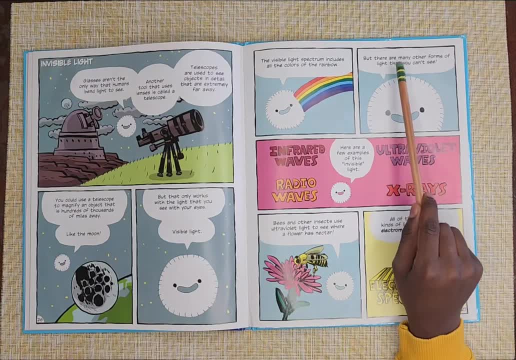 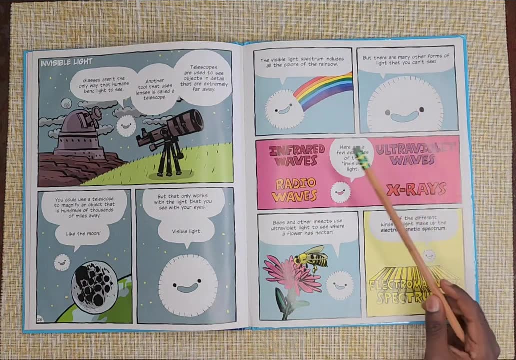 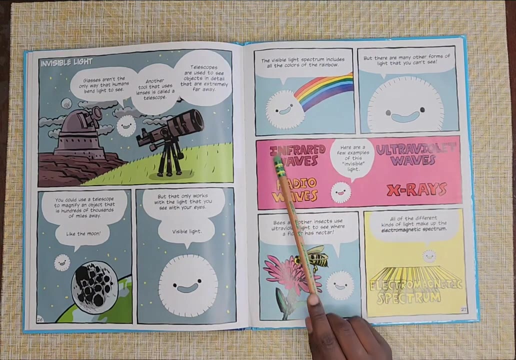 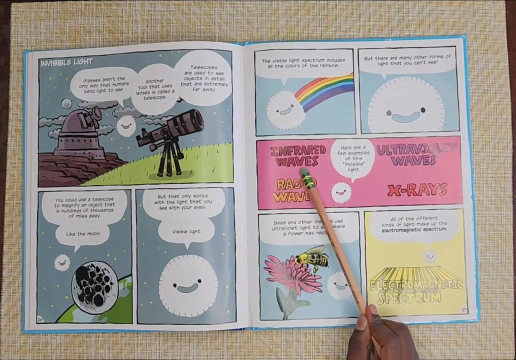 But there is. There are many other forms of light, Of light that you can't see. Here are a few examples of this: invisible light, Infrared light, Infrared waves, Infrared waves, Radio waves, Ultraviolet waves, X-rays. 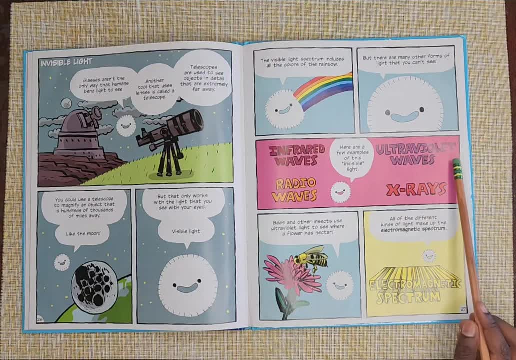 Like that tool that they use for checking your bones, And radio waves come from the radios. Ultraviolet Radio waves come from radios and also used for space, too. It comes from where they transmit messages and receive them. Ultraviolet waves Come from the sun. 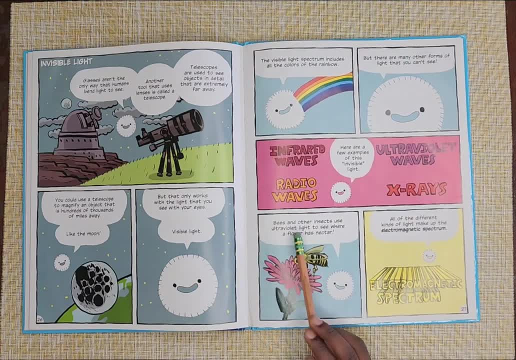 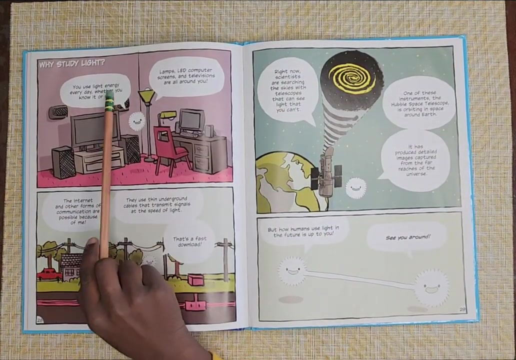 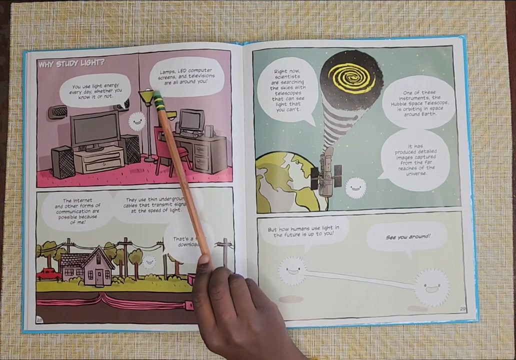 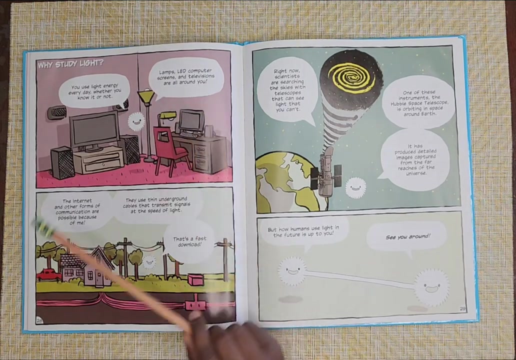 Bees and other insects use ultraviolet light to see where a flower has nectar. All of the different kinds of light make up the electromagnet spectrum. Why study light? You use light energy every day, whether you know it or not. Labs, LED computers, screens and television are all around you. 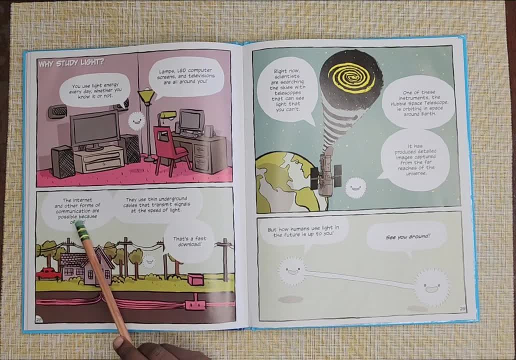 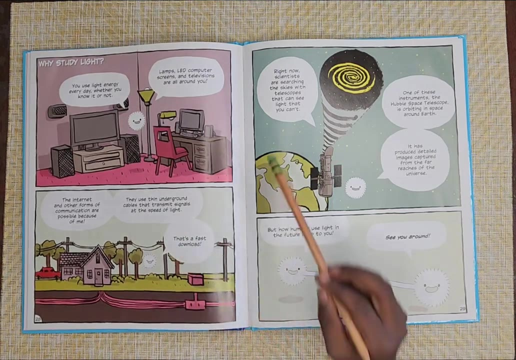 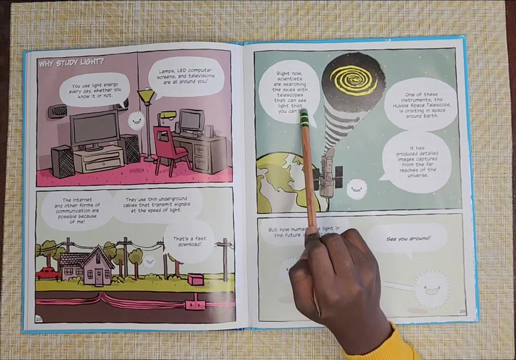 The internet and other forms of communication are possible because of me. They use thin underground cables that transmit signals at the speed of light. That's a fast download. Right now, scientists are searching the skies with telescopes that can't see light that you can't.